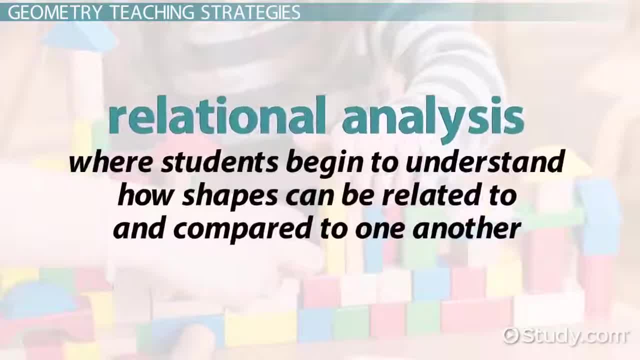 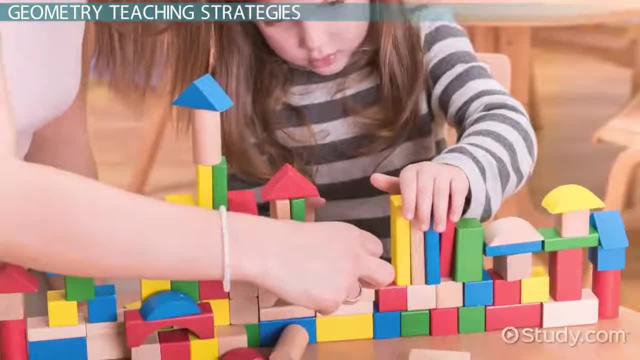 In addition, you want to introduce relational analysis where students begin to understand how shapes can be related to and compared to one another. You want them to understand that shapes can be above, below, behind, in front, larger, smaller, etc. 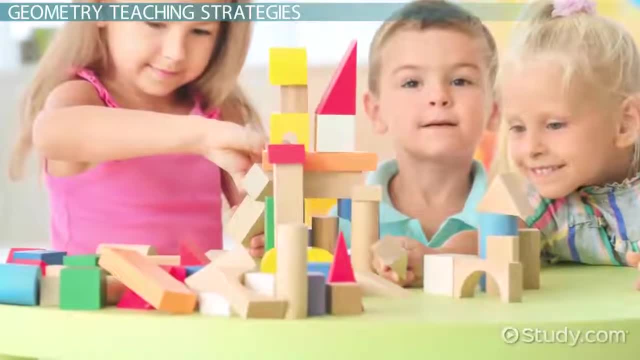 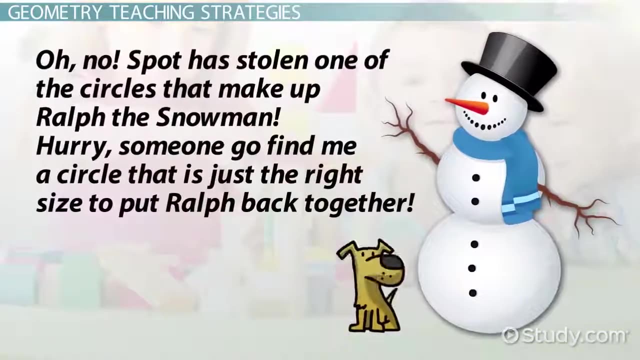 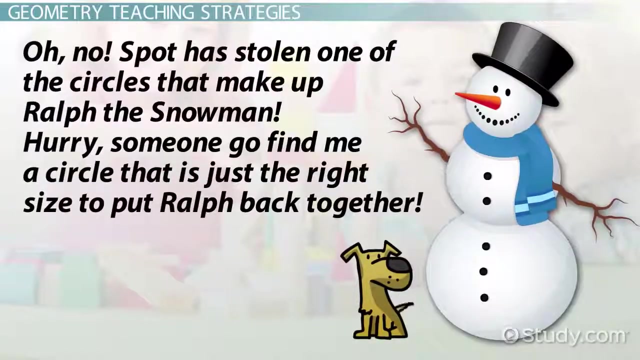 And how groups of them might look in relation to each other. For example, when introducing younger students to circles, you could provide them with the following scenario: Oh no, Spot has stolen one of the circles that make up Ralph the Snowman. Hurry, Someone, go find me a circle that's just the right size to put Ralph back together. 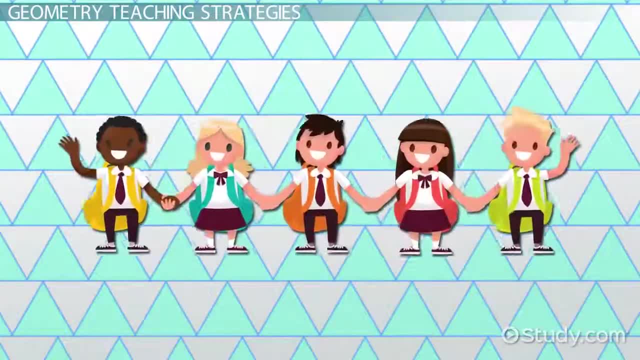 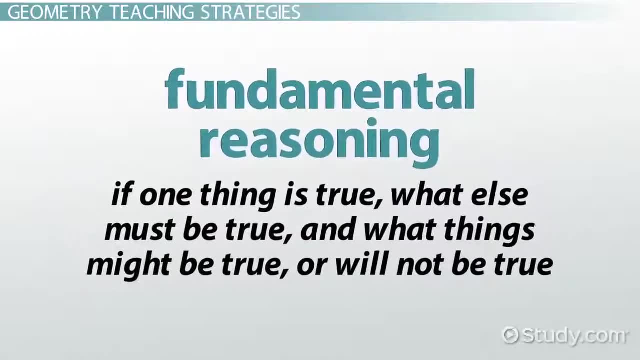 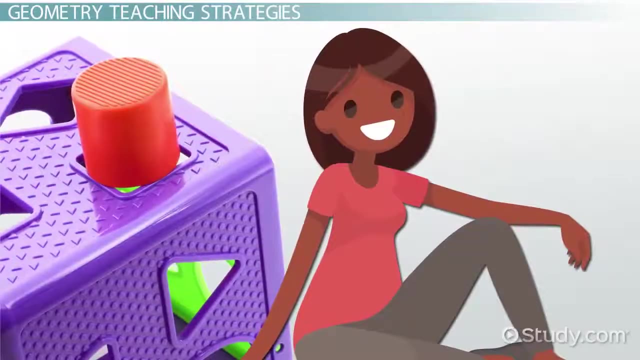 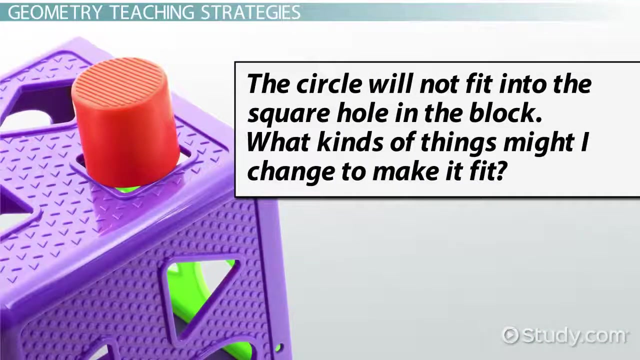 You also want to introduce patterns or the ways that shapes, numbers and other symbols can be meaningfully arranged, and fundamental reasoning, which means if one thing is true, you can change it. Finally, you want them to begin to understand problem-solving as it relates to shapes and patterns. For instance, the circle will not fit into the square hole in the block. What kinds of things might I change to make it fit? 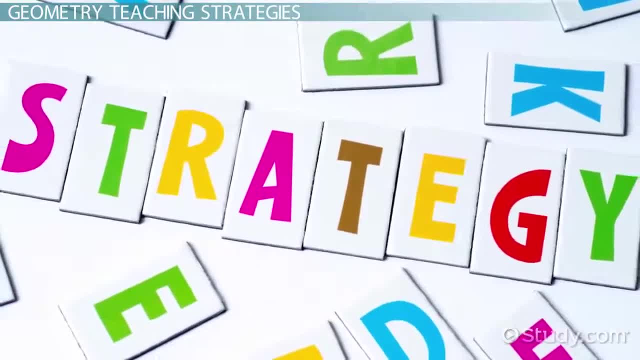 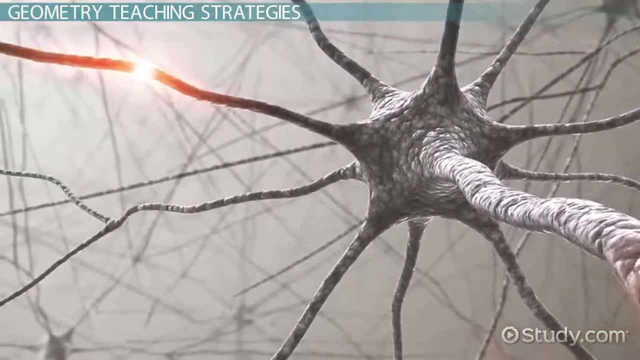 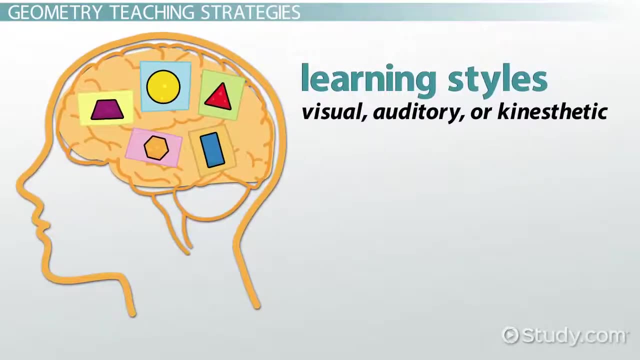 All strategies for meeting these objectives should involve several areas of the students' minds, because this reinforces their memory connections as they're learning. Lasting impressions are formed in the human mind, especially the young ones. one through the use of reinforcing sensory impressions, You want to appeal to as many learning styles, such as visual, auditory or kinesthetic. 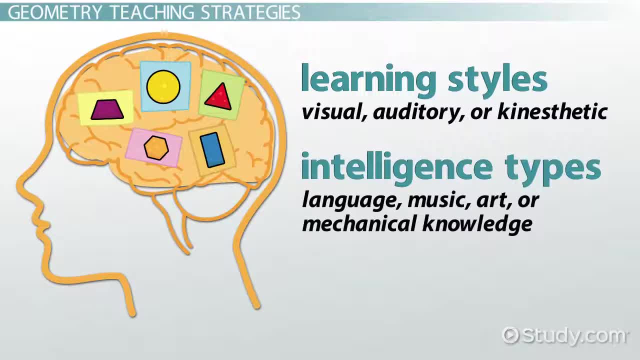 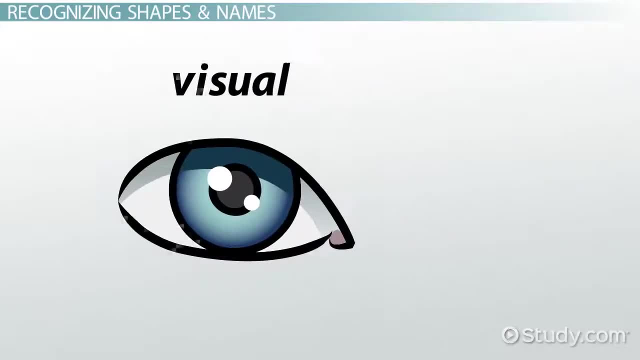 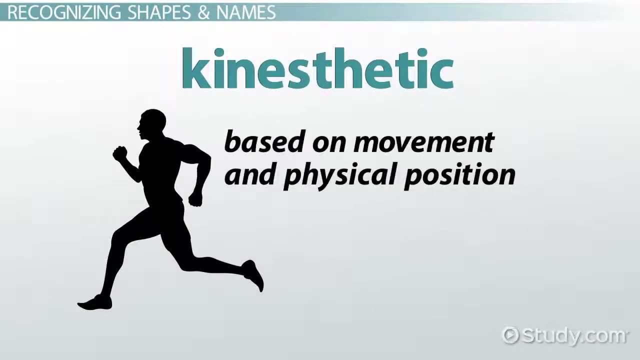 and intelligence types such as language, music, art or mechanical knowledge as possible. Combining drama with visual, auditory meaning based on language, sounds or music, and kinesthetic meaning based on movement and physical position components can create a memorable experience for your students. 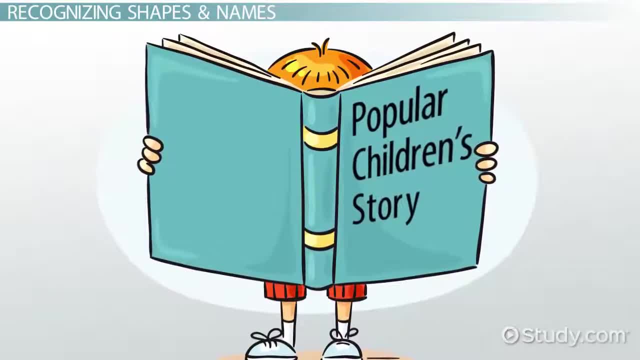 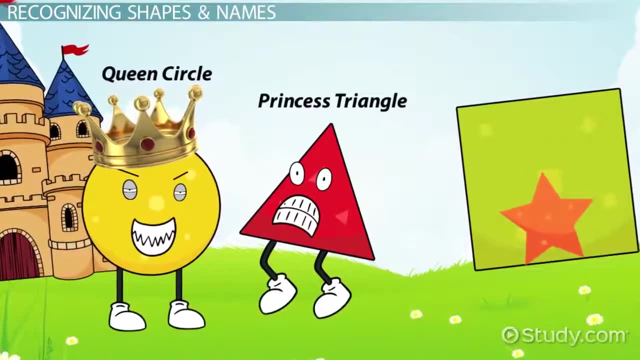 For example, any popular children's story can be retold and enacted using shapes for the main characters. You can tell the tale of how Queen Circle captured the poor Princess Triangle and imprisoned her in the large square with a small star-shaped door that only a star prince can go through. 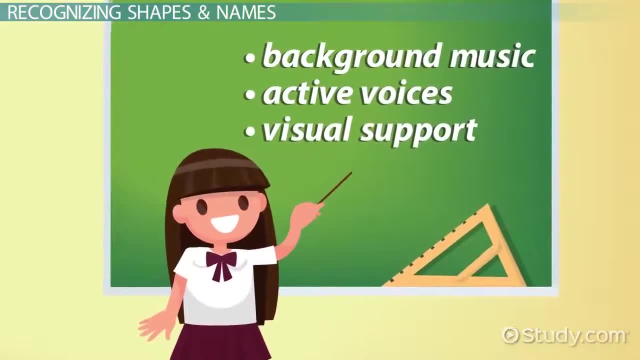 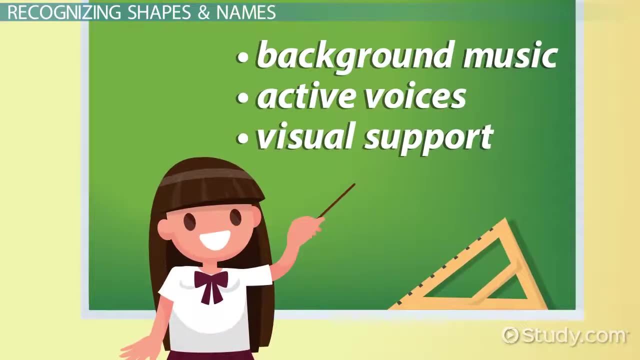 It can be pretty useful to have and use appropriate background music, active voices and visual support by way of large drawn, labeled and colored images for the set And for each of the actors and actresses to wear At key moments in the story. you can ask for clarification from the audience.